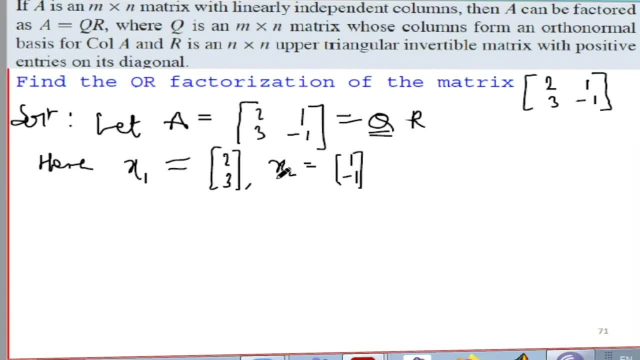 from this column vectors we construct the orthogonal basis for setting setting u1. u1 equals to x1, u1 equals to x1. where x1 is 2, 3, 2, 3 in column, but 2, 3, this is x1, but u2 is constructed. 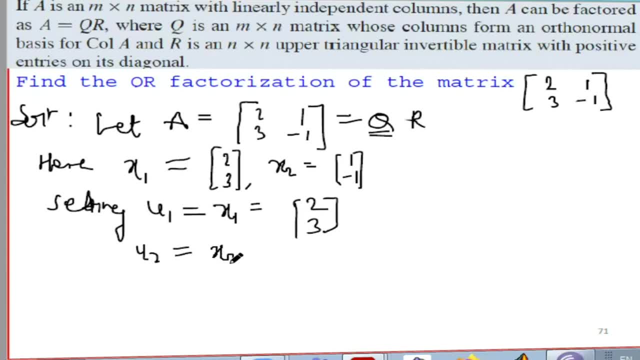 by the method uh. grammatical method: x2 minus x minus x2, dot, x2, dot, x1, x2, dot, x1, x1 means u1 and u1 dot, u1, u1, dot, u1, u1, u1. by this method, granite is constant and here u2, x2, x2 is 1 minus 1, 1, 2, 1 minus 1, u1 is also x1. 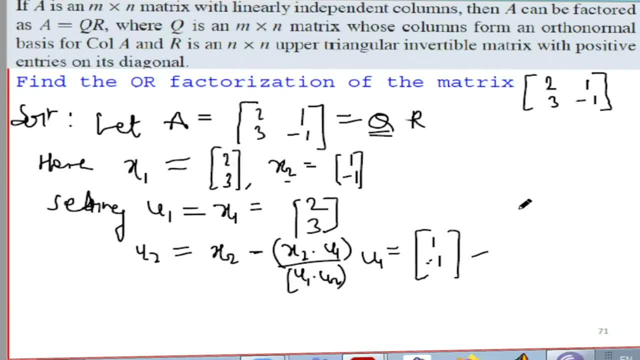 so dot product of these two vectors, 2 into 1, 2 and 3 into minus 1 minus 3. so 2 minus 3, 2 minus 3. divide by u1 dot. u1: u1 is x1, x1 dot. x1 is 2 to the 4 plus 3 to the 9.. this is the dot product. 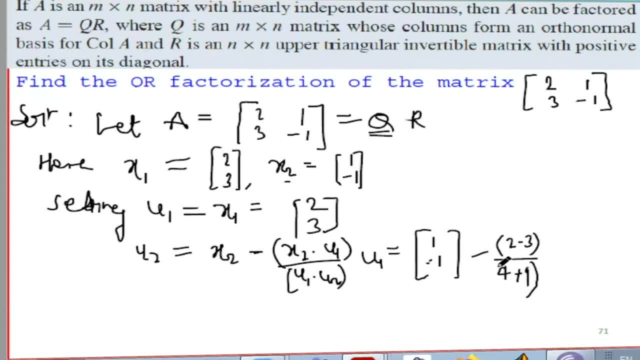 of u1 and u1, 4 plus 9 and u1. the u1 vector is x1, which is 2, 3. this is u2, so ut is 1, 1. 1. 1 is here of minus 2 minus 3. 2 minus 3 is minus 1 plus 1 by 1 by 9 plus 4, 13. 1 by 13. 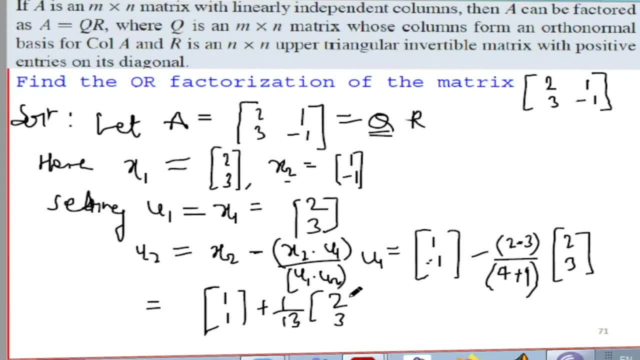 or 2, 3. this equals to 1 minus 1, 0. x2 is 1 minus 1. 1 by 13, 2, 2 by 13 plus 1, 2 by 13 plus 1. 13 to 15, 15 by 13. 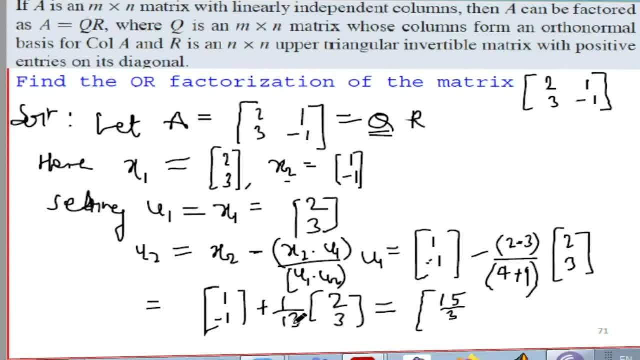 15 by 13 and 3 by 13 minus 1 by 13.. minus 10, 10 divide by 13.. this is u2. this u1 and u2 are orthogonal basis for calling a orthogonal. from this orthogonal basis we construct ortho normal. 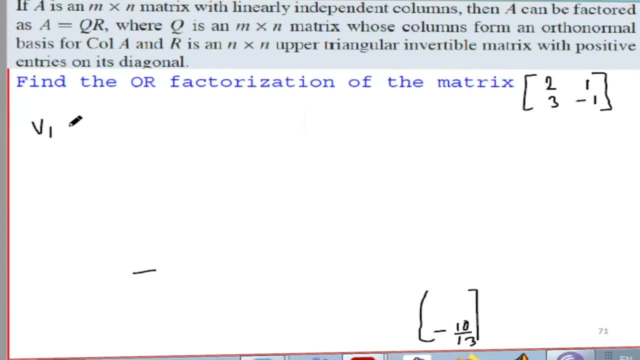 we write: b1 is orthonormal b1. norm of u1. this is orthonorm. so u1 is 2, 3 and the norm of u1, norm of u1 is root over 2 to the 4 to 2, this 4, this 2 to the 4 and 3, 9, 2 plus 9 is 14.. 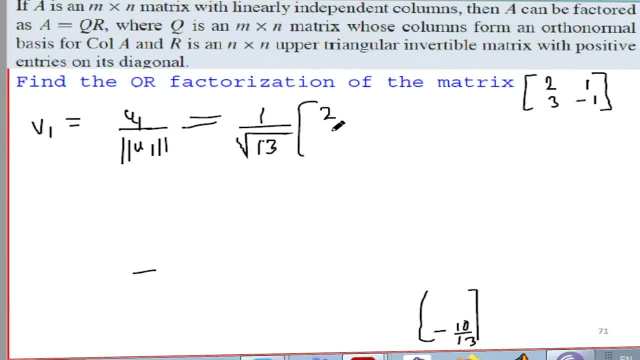 and u1. u1 is 2, 3. this is u1 orthonormal b1. So V2 equals to U2 divided by norm of U2.. The orthonormal vectors is constructed from orthogonal vectors. U1 and U2 are orthogonals. 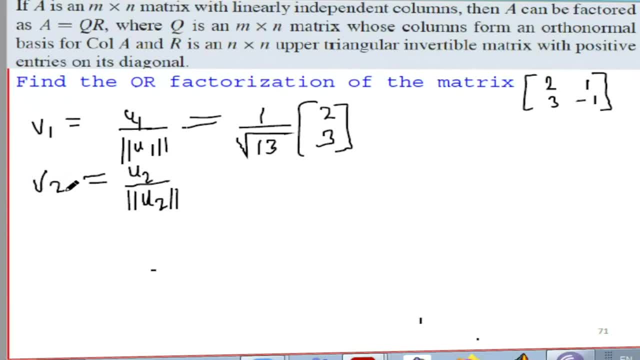 Here V2 and V1 are orthogonal. This equals to V2.. V2 means 15 by 13, equals to 15 by 13.. This U2, this U2 is minus 10 by 13,, minus 10 by 13.. 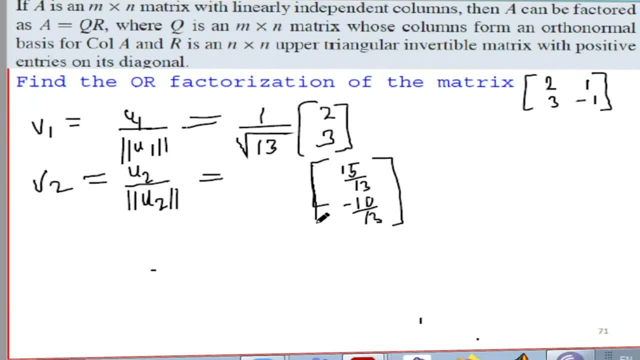 This is U2.. And its norm. norm is square root of 15 by 13 whole square, plus minus 10 by 13 whole square, So that 1 by square root of 15 by 13 square plus minus 10 by 13 square. 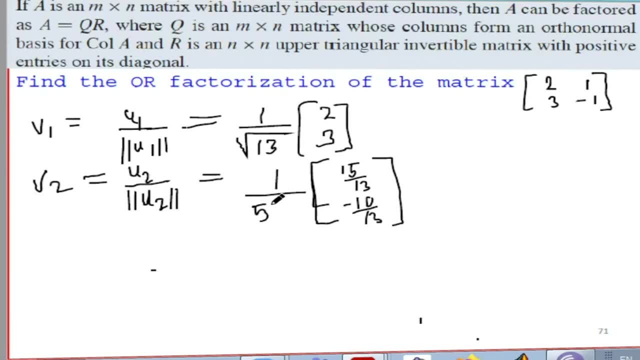 Equals to 5 root 13, root 13 by 13.. This is the norm of U2.. Norm of U2 means the square root of 15 by 13 whole square, plus minus 10 by 13 whole square, Which is equal to 13 by 5 root 13.. 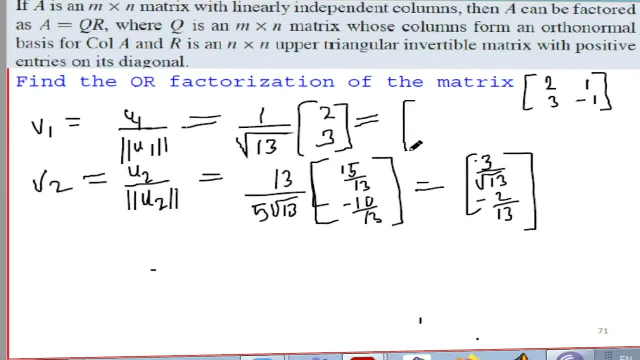 And V1,. V1 is 2 by root 13,, 2 by root 13. And 3 by root 13,, 2 by root 13.. In this way we construct Q. The Q is orthonormal basis for column A. 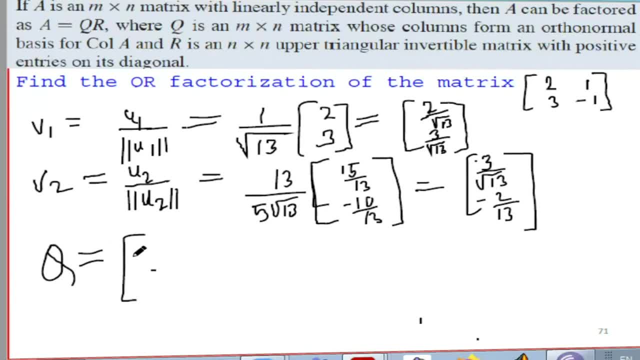 So this Q vector, Q vector, the Q matrix is 2 by root 13,, 2 by root 13, and 3 by root 13,, 3 by root 13.. And V2, 3 by root 13,, 3 by root 13,, minus 2 by root 13.. 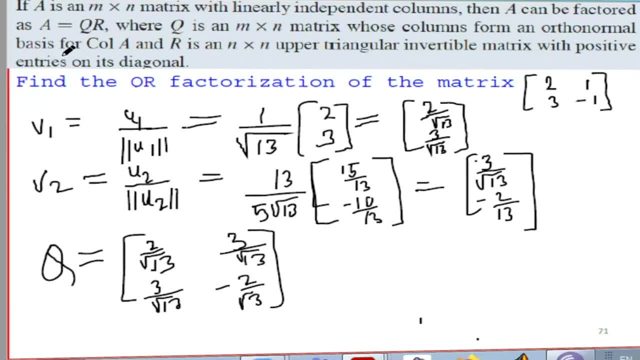 This is Q, So PA can. but PA can be characterized as Q into R. The R vector is the upper triangular vector which is obtained by the formula, the transpose of Q into A, So transpose of Q. Q transpose means its transpose. 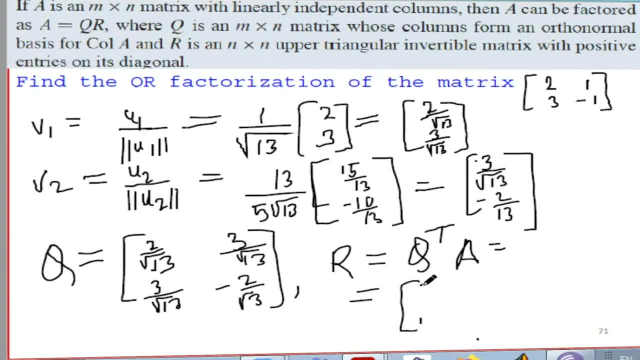 Its transpose is 2. by transpose of Q And A, A equals to given matrix. A is the given matrix is 2, 3, and 1, minus 1.. So multiplying these two matrices, It's minus 6 plus 6, 0.. 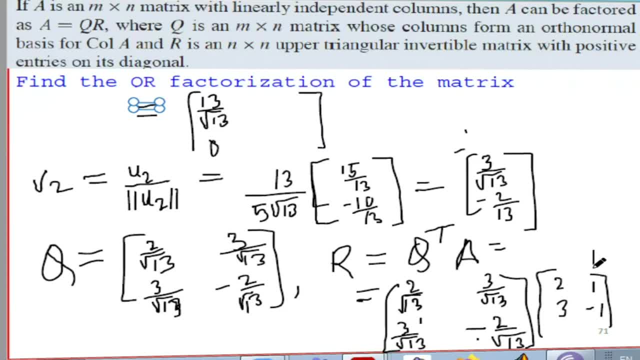 And this second row, second column. this multiplied first row of the first matrix and second row of the first matrix. So this second column, 1 minus 1.. 1 is multiplied to 2 by root 13,, 2 by root 13, and minus 1 is multiplied by 3 by root 13.. 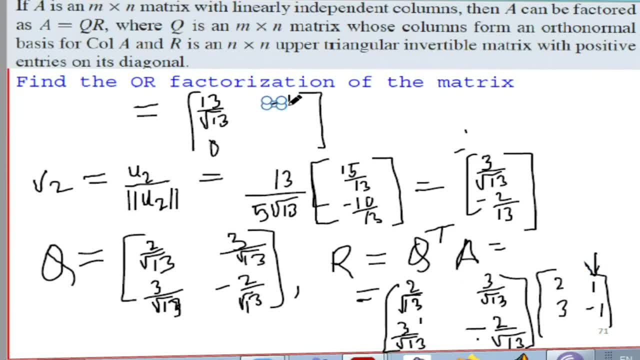 2 minus 1.. Minus 3 equals to minus 1.. Minus 1 by root 13.. Minus 1 by root 13 is this column: And if this multiply in the second row 1 into 3, 3, and minus 1 into minus 2 plus 2.. 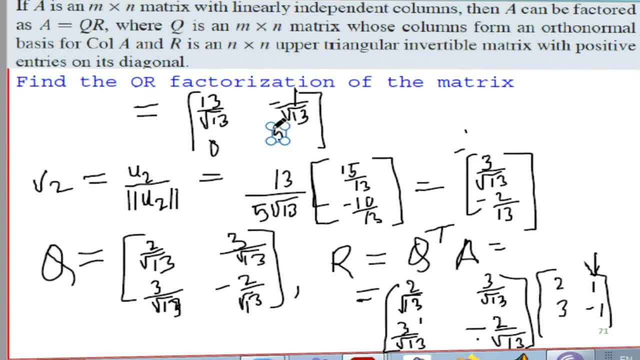 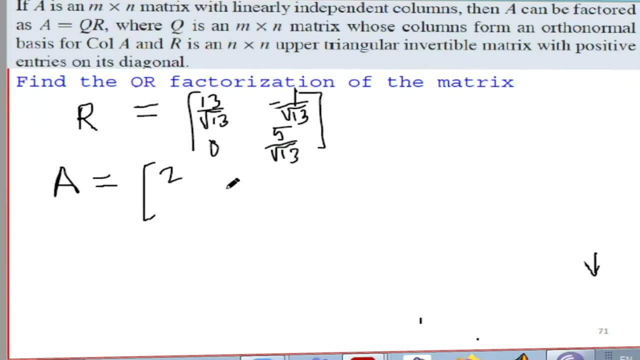 So 3 plus 2, 5.. 5 by root 13.. 5 by root 13.. This is the R matrix, which is upper triangular matrix, So A. So A is 2, 3,, 2,, 2, 3, and 1, 1, minus 1..